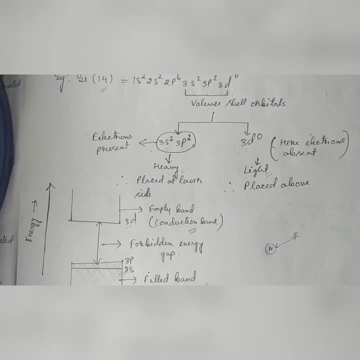 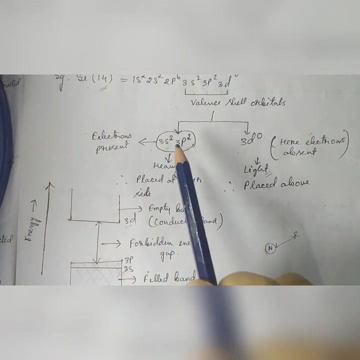 So here there are two types of valence bands. The first one is that this 3s and 3b Orbitals, which have electrons, and this orbital 3d, which doesn't have electrons. Yes, so because of having electrons, these orbitals are heavy, and because this orbital is empty, therefore this orbital is light. Yes, since these orbitals are heavy, that's why they are placed at the lower side, and since they are light, and therefore they are placed at upper side or placed above, Yes, 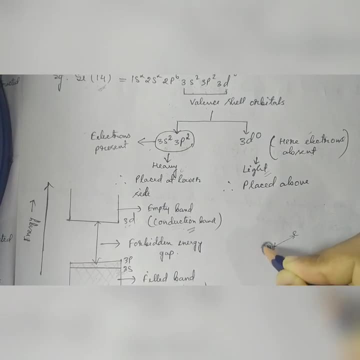 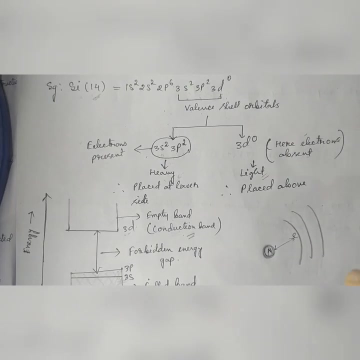 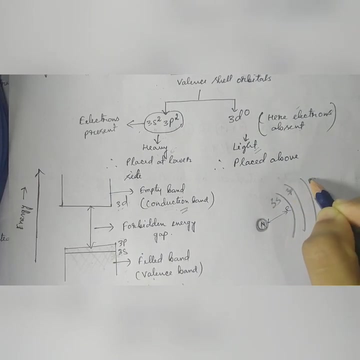 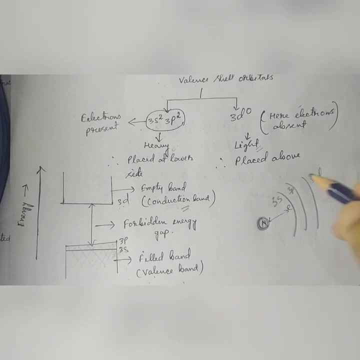 Now, let us take this as what this? let us take this is what nucleus, and we know that electrons are revolved around the nucleus. So so this band is for 3s, This is for 3p and this is 3d. Yes, Now we know that here the 3s and 3p orbital have what electrons, So there will be a attractive force between these electrons. 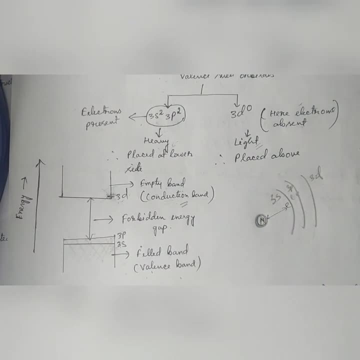 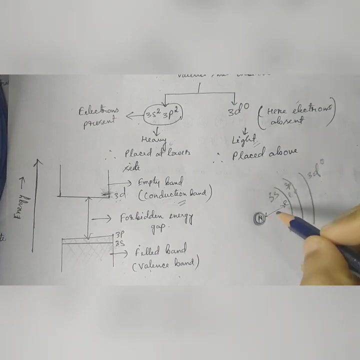 With this nucleus. Yes, So it will pull these orbitals towards itself. Therefore, these orbitals will be placed at the lower side. Now, here 3d is zero. That means there is no electrons in 3d orbital. That's why there will be no attractive force between these nucleus with this 3d orbital. Yes, So this 3d will be a little bit far from this 3s and 3p. 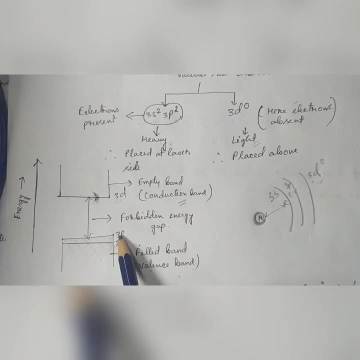 With this nucleus, the electrons are pressed at the lower side of this 3d orbital. So this is the band of 3s and this is 3p And this is man forward Three. Now this three dependent is empty. There is nothing. So this empty fromavour Wheat conduction band, and hear this. 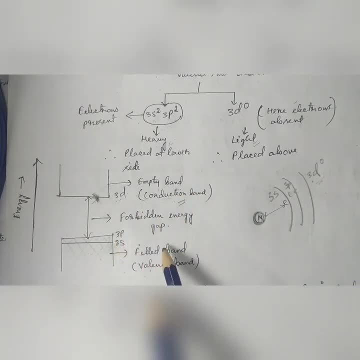 On this. 3s and 3p Bands are filled with electrons, and this field bands are known as balanced bands. There is a energy gap between this conduction band, the valence band. this gap is known as what forbidden energy gap. so, conductors, 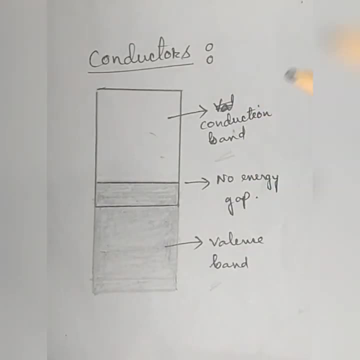 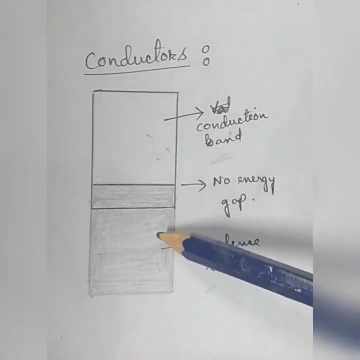 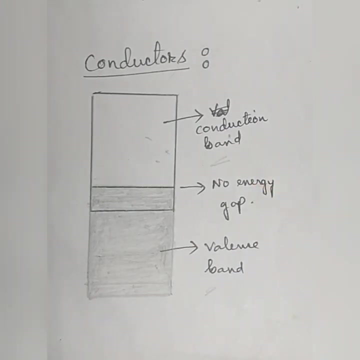 so what is conductors? so in conductors, the conduction band and the valence band- that means the empty band and the field bands- are overlap with each other. okay, there is no energy gap between this conduction band and valence band. therefore, the electrons of this field band can jump easily to the 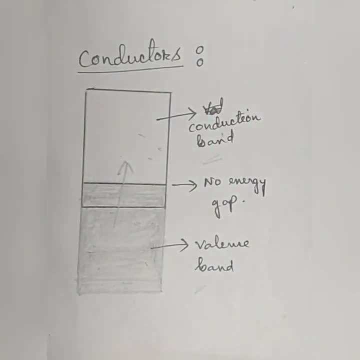 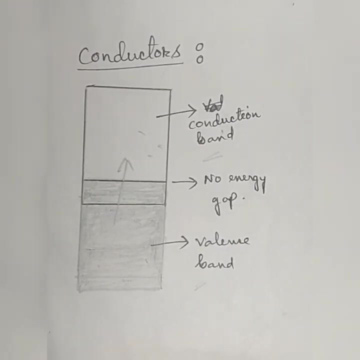 conduction band. okay, and we know that when electron electrons move from one place to another, then electricity is generated. so a conductors can generate electricity easily, because here the movement of electron is easy, since there is no energy gap between the conduction band and valence band. 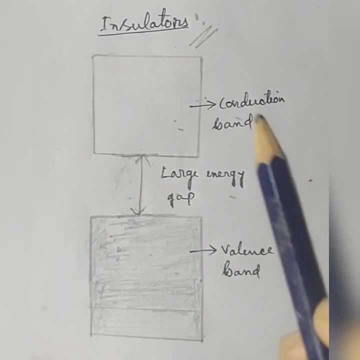 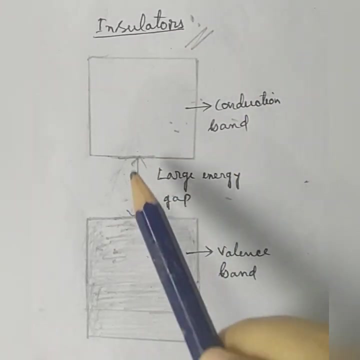 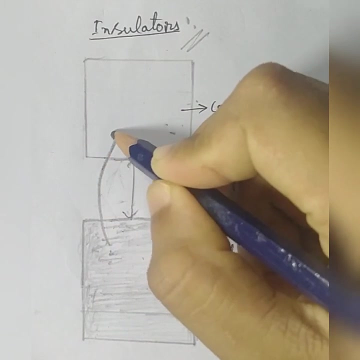 so next one is what insulators? okay, so what happen in insulators? so this one is what conduction band and this one is what valence band. in case of the insulator, the energy gap between this valence band and conduction band is very large, so the electron of this valence band cannot jump to the conduction. 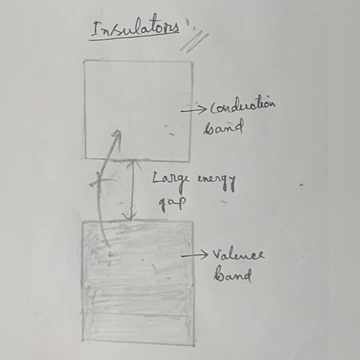 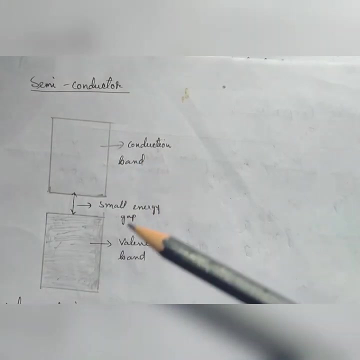 band. okay, so there is no flow of electron. that means they cannot conduct electricity. that means they have a very small electrical conductivity. next one is semiconductor in semiconductor. the energy gap between this conduction band and the valence band is what? very small. that's why some 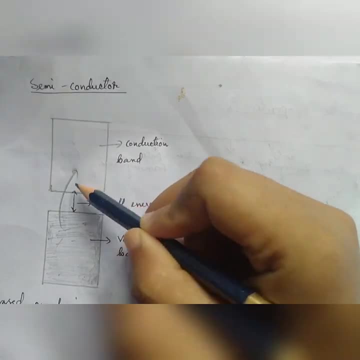 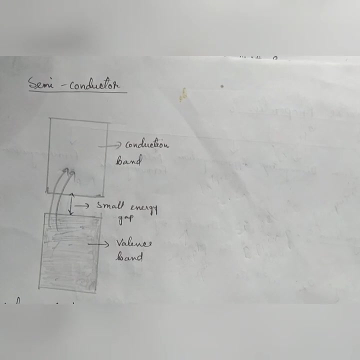 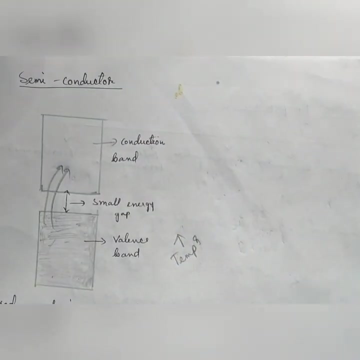 amount of electron from this valence band can jump to the conduction band. okay, so movement of electron means what they can conduct, electricity. okay now, if you increase the temperature. okay now, if you increase the temperature, then the movement of electron will be more, yes or no. so more of the electron will now jump to the conduction band and because of this, 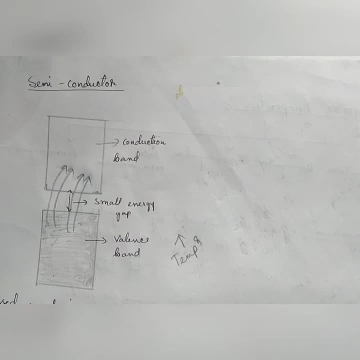 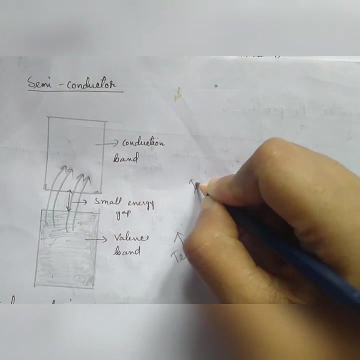 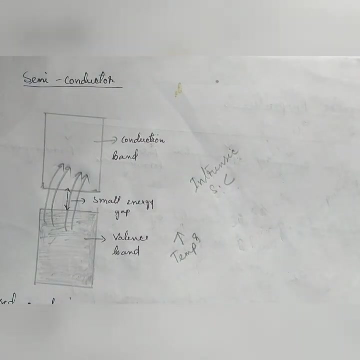 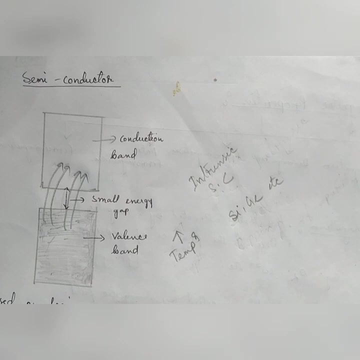 movement, the electrical conductivity will increase more. okay, and because of this reason semiconductor are again also known as what intrinsic semiconductors? okay, and the substances like silicon, silicon, germanium, etc. show the behavior of semiconductors. okay, now again, the electrical conductivity of semiconductor can be increased by the process called doping. okay, you already know what is doping. 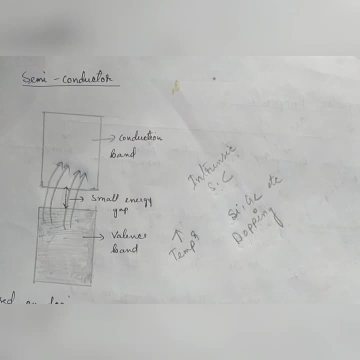 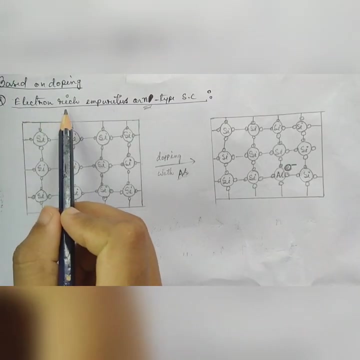 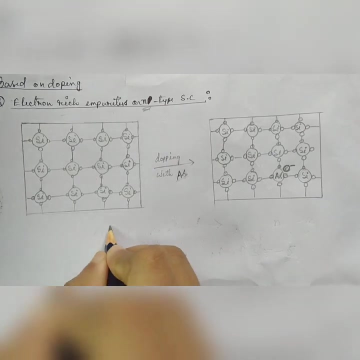 doping means the addition of impurity or mixing of impurity. so by this process also we can increase the electrical conductivity of a semiconductor. semiconductors is on doping. semiconductors are classified into two parts. the first one is what electron rich impurities or n-type semiconductors. so in n-type semiconductor group. 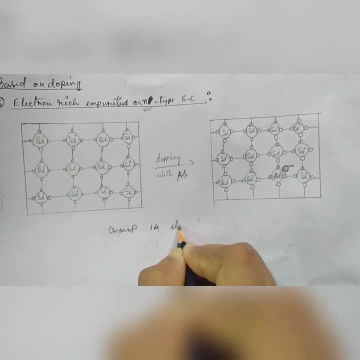 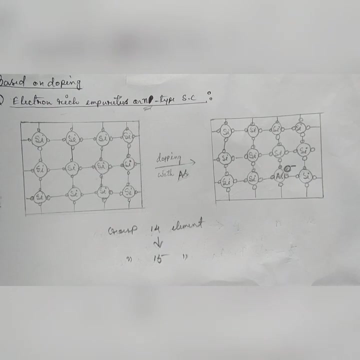 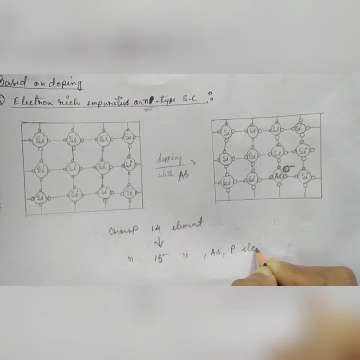 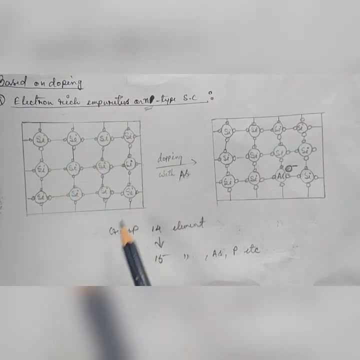 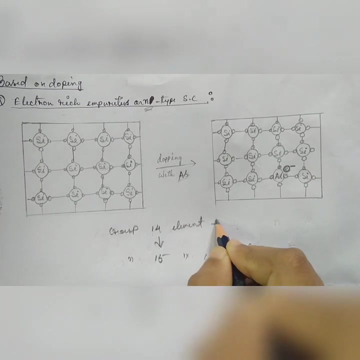 14 elements are doped with group 15 elements. okay, group 14 elements are doped with group 15 elements, for example, for example, arsenic, phosphorous, etc. okay, so for this type of semiconductor, we took the perfect crystal of a group 14 element, that is, silicon, because silicon is a group 14 element. and in case of group 14 elements, 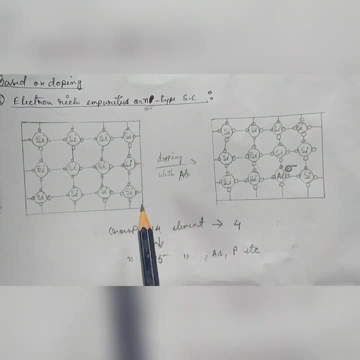 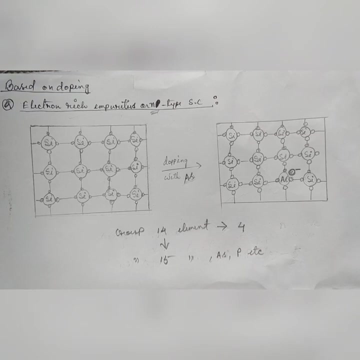 there are total four valence electrons are there. so silicon has a four valence electron: one, two, three, four. one, two, three, four. so they. so this silicon has how many. so this silicon has how many valential electron: one, two, three, four. this silicon has also one, two. 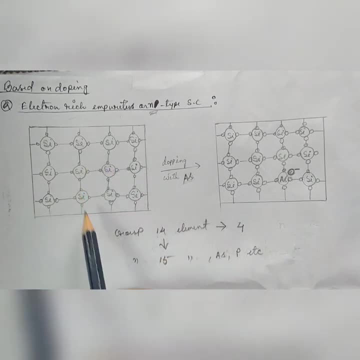 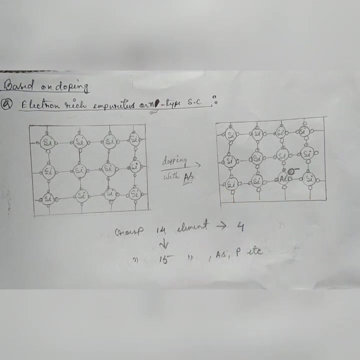 three, four, so they will form a bond with each other to create this perfect crystal. now this silicon will dope with arsenic or phosphorus, that means with the group 15 element. okay. now in group 15 element there are total five number of valence electrons. are there, okay? so let us replace this. 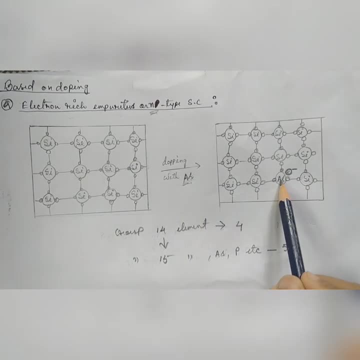 silicon with this arsenic. okay, so we replace here and what we say there are total five valence electrons in case of the arsenic, one, two, three, four, five. okay, now this four electrons: one, two, three, four. they will use in the formation of a covalent bond. 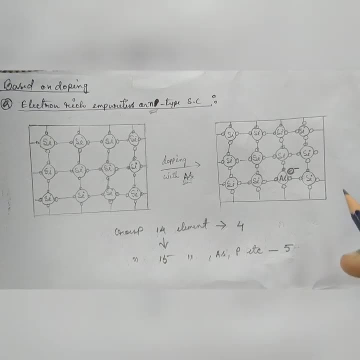 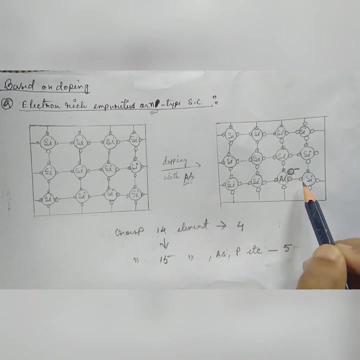 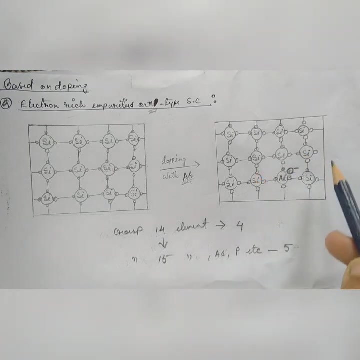 with its neighboring silicon elements. Okay, but the fifth number of electrons is remains as what extra. and this is free here because it is not bonded with any type of atoms or with any electrons. so here this electron is free, so they will delocalized in this crystal. that means electrons. 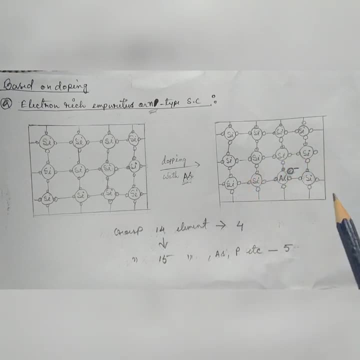 will move in this crystal. now what we got? that when electron moves, then they generates what electricity? so because of this, the localization, the electrical conductivity will increase okay. the electrical conductivity of dope silicon will increase okay, and this increase is because of this negative charge, electron. that's why this is also known as what n. 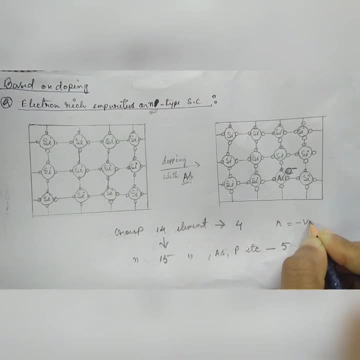 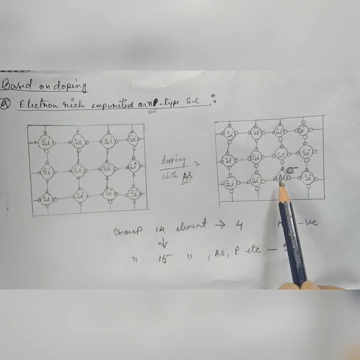 type semiconductor. here n is for negative charge and this is electron reach, because here the number of electron increases, as before, because arsenic has five valence electron but silicon has only four valence electrons, so electron is increase as compared to the first crystal. okay, the second type. 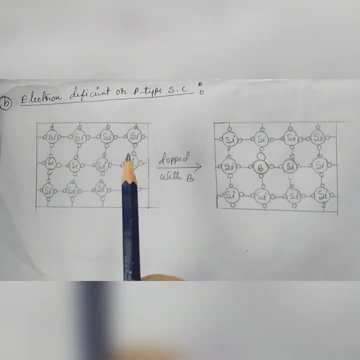 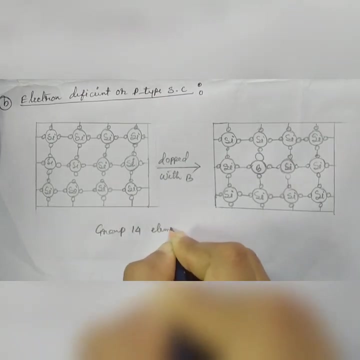 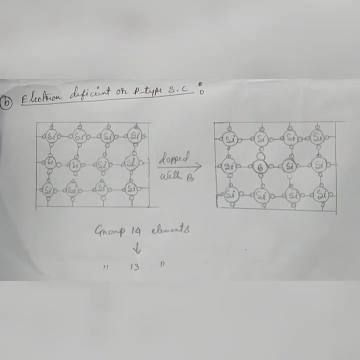 is electron deficient or p-type semiconductor. in p-type semiconductor, group group 14 elements are dope with group 13 elements. okay. group 14 elements are dope with group 13 elements. okay. group 14 elements are dope with group 13 elements. okay. so here also we took the. 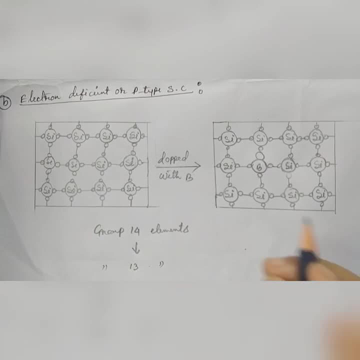 so here also we took the. so here also we took the crystal of silicon, because here silicon is crystal of silicon, because here silicon is crystal of silicon, because here silicon is one group 14 element, and we know that one group, 14 element, and we know that. 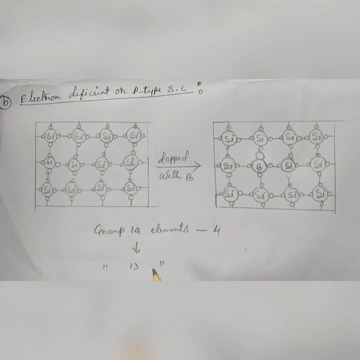 one group 14 element and we know that in group 14 element there are total four. in group 14 element there are total four. in group 14 element there are total four valence electrons and in case of the valence electrons and in case of the 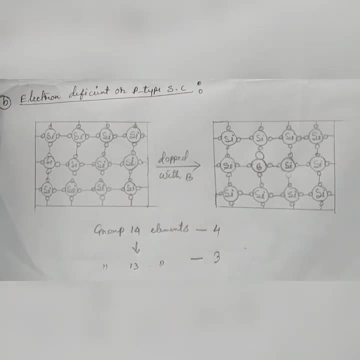 valence electrons and in case of the group 13 elements, there are total three group 13 elements. there are total three group 13 elements. there are total three valence electrons. are there? okay, now for valence electrons. are there? okay, now for valence electrons. are there? okay now, for example, boron, aluminium, etc. these are 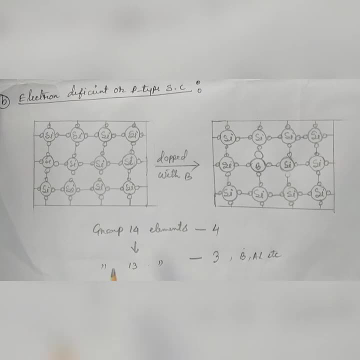 example, boron, aluminium, etc. these are example: boron, aluminium, etc. these are what group 13 elements? okay, now this. what group 13 elements? okay, now this. what group 13 elements? okay now. this crystal will drop with group 13 element. crystal will drop with group 13 element. 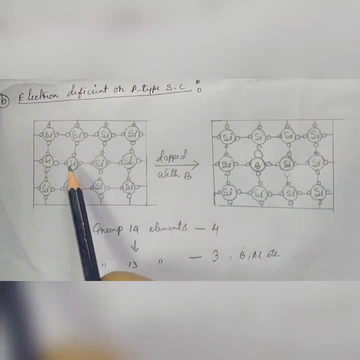 crystal will drop with group 13 element. say boron okay, so we replace this. say boron okay, so we replace this. say boron okay, so we replace this. silicon with one of the boron atom and silicon with one of the boron atom and silicon with one of the boron atom. and what we said in group 13 element there. 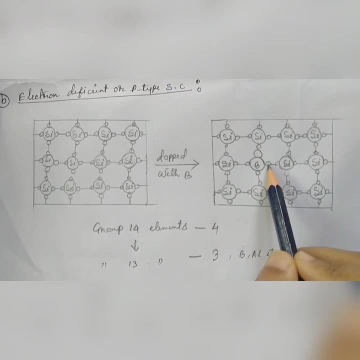 what we said in group 13 element. there, what we said in group 13 element, there are only three electrons: one, two, three are only three electrons: one, two, three are only three electrons: one, two, three. okay, so at first these three electrons. okay, so at first these three electrons. 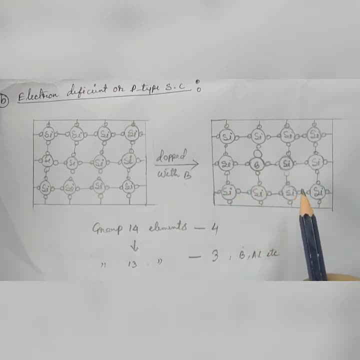 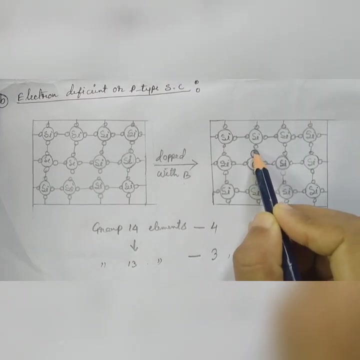 okay. so at first, these three electrons will participate in the formation of bond. will participate in the formation of bond. will participate in the formation of bond with this neighboring silicon atoms- okay, with this neighboring silicon atoms. okay, with this neighboring silicon atoms, okay. and this place is what electron hole that? 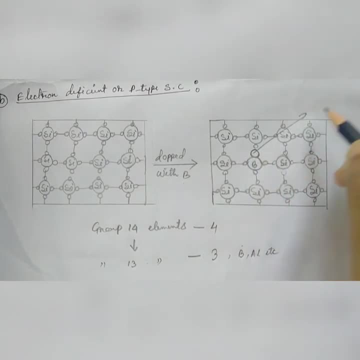 and this place is what electron hole. that and this place is what electron hole. that means this: a boron atom will create one. means this: a boron atom will create one. means this: a boron atom will create one of the electron hole this hole will, of the electron hole, this hole will. 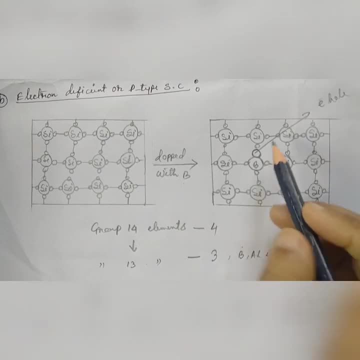 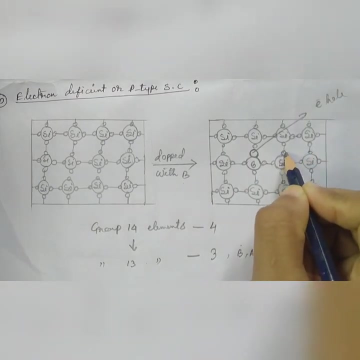 of the electron hole, this hole will generate automatically. okay now, since generate automatically. okay now, since generate automatically. okay now, since this is whole. that means what this is a. this is whole. that means what this is a. this is whole. that means what this is: a free space. okay, so this electron now will. 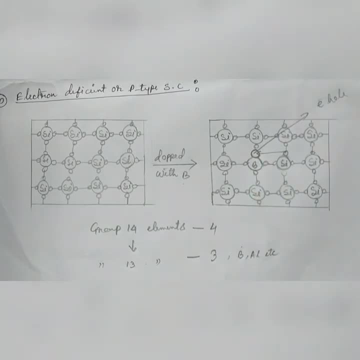 free space. okay, so this electron now will free space. okay, so this electron now will try to try to try to move towards this hole. okay now, if this move towards this hole. okay now if this move towards this hole. okay now if this electron moves to this. hold an electron. 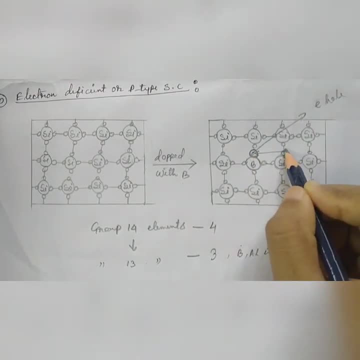 electron moves to this hold an electron, electron moves to this hold an electron will come here and this place will now will come here and this place will now. will come here and this place will now. create what new one? okay, this position. create what new one? okay, this position. 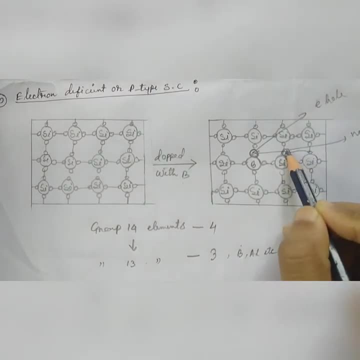 create. what new one? okay, this position is now. what new hole again? this electron is now. what new hole again? this electron is now. what new hole again? this electron will go to or move towards this hole and will go to or move towards this hole and will go to or move towards this hole and electron will be come here and this. 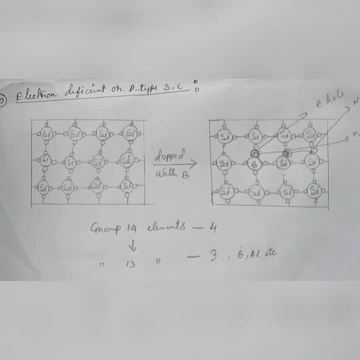 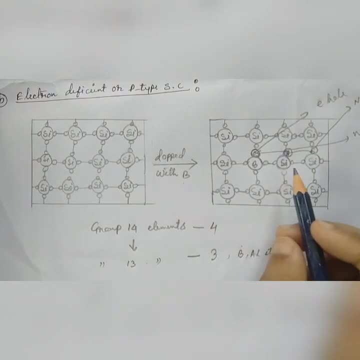 new hole. okay so, and the process will be continue like this. so the movement or the continue like this. so the movement or the continue like this. so the movement or the direction of the electron is in which direction of the electron is in which direction of the electron is in which direction direction of electron is in. 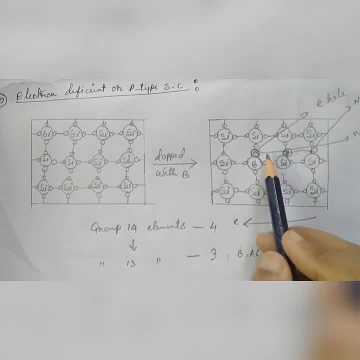 direction: direction of electron is in direction, direction of electron is in this direction, and the direction of this, this direction, and the direction of this, this direction, and the direction of this hole, electron hole is in which direction hole, electron hole is in which direction hole, electron hole is in which direction? in this direction. so this will be the 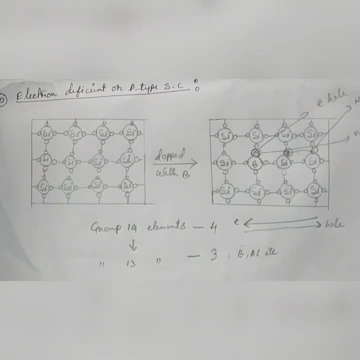 in this direction, so this will be the in this direction, so this will be the direction of hole. okay, now, this is what direction of hole. okay, now, this is what direction of hole. okay, now, this is what. electron deficient, now electron. electron deficient, now electron. electron deficient, now electron deficient means what when we consider: deficient means what when we consider deficient means what when we consider positive, positive means. what electron positive, positive means, what electron positive, positive means, what electron deficient and negative means, what deficient and negative means, what deficient and negative means, what electron reach, so here in semiconductor. electron reach, so here in semiconductor. 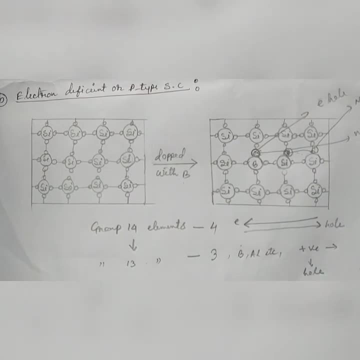 electron reach. so here in semiconductor this positive is considered as what hole. this positive is considered as what hole. this positive is considered as what hole. okay, so this whole of electron will be okay. so this whole of electron will be okay. so this whole of electron will be considered as what positive hole. okay now. 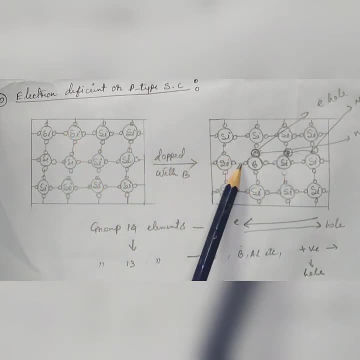 considered as what positive hole. okay, now, considered as what positive hole. okay now. here the number of electron will decrease. here the number of electron will decrease. here the number of electron will decrease because boron has only three valence. because boron has only three valence. 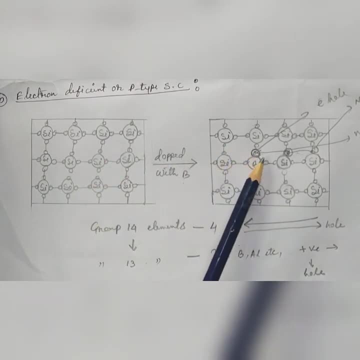 because boron has only three valence electron but silicon has four valence electron, but silicon has four valence electron but silicon has four valence electron. so one of the electron is less electron, so one of the electron is less electron. so one of the electron is less in this crystal as compared to this. 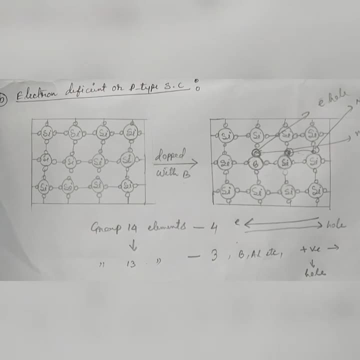 in this crystal, as compared to this, in this crystal, as compared to this crystal. therefore, this is what electron crystal. therefore, this is what electron crystal. therefore, this is what electron deficient, and this is called P type of deficient and this is called P type of deficient and this is called P type of semiconductor. P is, for this, positive. 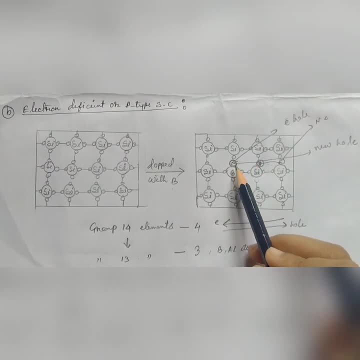 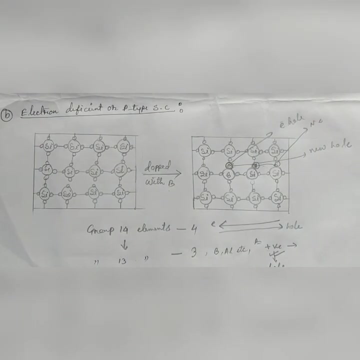 semiconductor P is for this positive semiconductor, P is for this positive church. okay, cause of this hole, the church. okay, cause of this hole, the church. okay, cause of this hole, the electrons can move. yes, so movement of electrons can move. yes, so movement of electrons can move. yes, so movement of production of electricity. that means 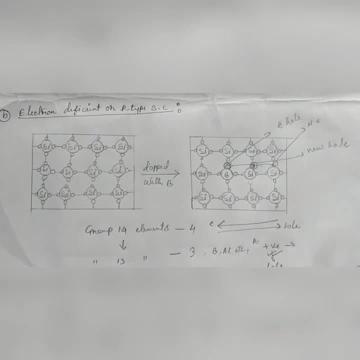 production of electricity. that means production of electricity. that means because of this hole, the electrical, because of this hole, the electrical, because of this hole, the electrical conductivity of this crystal will conductivity of this crystal will conductivity of this crystal will increase magnetic properties of solids, increase magnetic properties of solids. 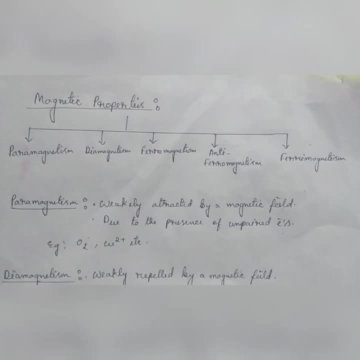 increase magnetic properties of solids. the magnetic properties of solids are the magnetic properties of solids are the magnetic properties of solids are classified into five parts: paramagnetism classified into five parts. paramagnetism classified into five parts. paramagnetism, diamagnetism, ferromagnetism. 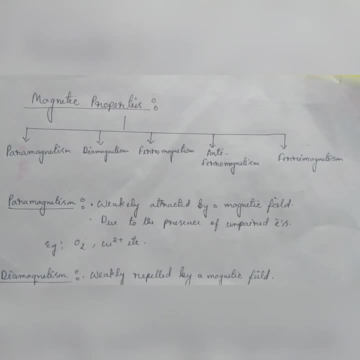 diamagnetism, ferromagnetism, diamagnetism, ferromagnetism, antiferromagnetism and very magnetism, antiferromagnetism and very magnetism, antiferromagnetism and very magnetism. let's discuss one by one. first one is: let's discuss one by one. first one is: 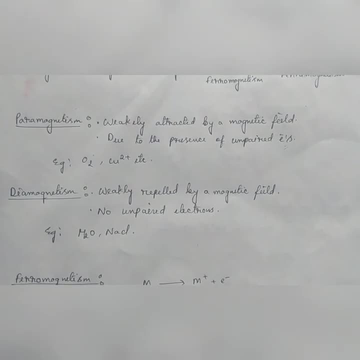 let's discuss one by one. first one is paramagnetism, so paramagnetism, are those: paramagnetism, so paramagnetism, are those paramagnetism, so paramagnetism. are those substances which are weakly attracted by substances which are weakly attracted by substances which are weakly attracted by a magnetic field when applied in a 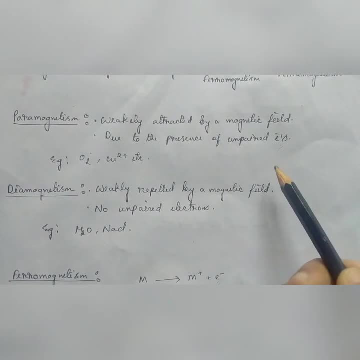 a magnetic field when applied in a. a magnetic field when applied in a magnetic field, and this is due to the magnetic field, and this is due to the magnetic field, and this is due to the presence of unpaired electron, okay, and presence of unpaired electron, okay, and 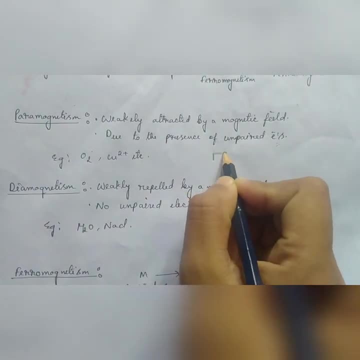 presence of unpaired electron. okay, and now suppose unpaired electron means what. now suppose unpaired electron means what. now suppose unpaired electron means what? in orbital they will be present like this: in orbital they will be present like this: in orbital they will be present like this: these are what, unpaired electron. so 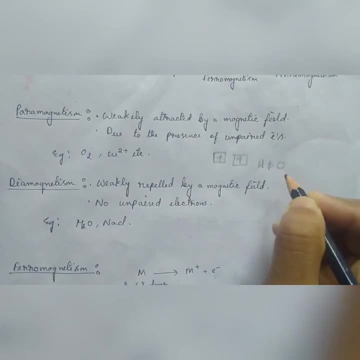 these are what unpaired electron. so these are what unpaired electron. so here the magnetic moment will be not here. the magnetic moment will be not here. the magnetic moment will be not equal to zero because no direction is in. equal to zero because no direction is in. 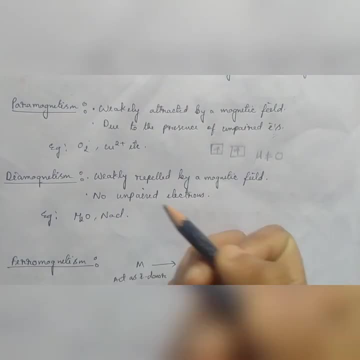 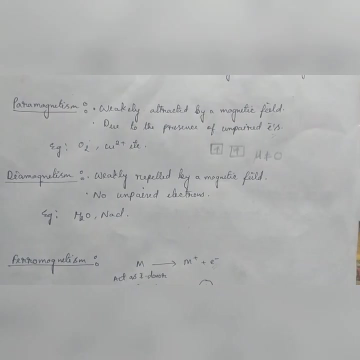 equal to zero, because no direction is in the same direction. okay, example o2: the same direction. okay, example o2- the same direction. okay, example o2: copper to, et cetera. we already studied copper to, et cetera. we already studied copper to, et cetera. we already studied, in element that the o2 molecule has what 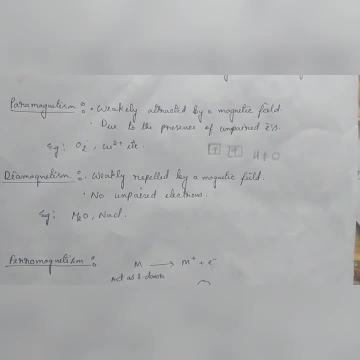 in element that the o2 molecule has. what in element that the o2 molecule has? what unpaired electron. likewise copper 2- unpaired electron. likewise copper 2 unpaired electron. likewise copper 2. plus has also unpaired electron, so they are. plus has also unpaired electron, so they are. 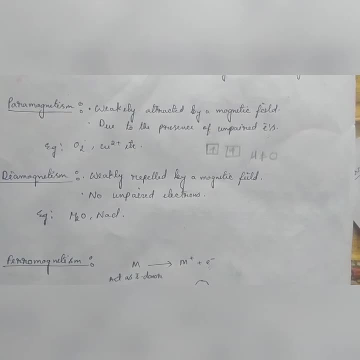 plus has also unpaired electron. so they are known as what paramagnetism now. next known as what paramagnetism now. next known as what paramagnetism now. next one is for diamagnetism now those. one is for diamagnetism now. those one is for diamagnetism now, those substances which so diamagnetism are. 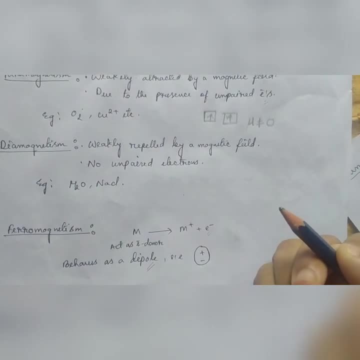 substances which so diamagnetism are substances which so diamagnetism are weakly repelled by a magnetic field. okay, weakly repelled by a magnetic field. okay, weakly repelled by a magnetic field. okay, and they doesn't have unpaired electrons. and they doesn't have unpaired electrons. 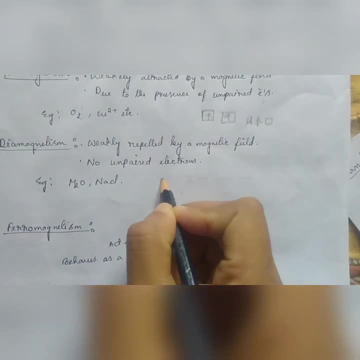 and they doesn't have unpaired electrons now and doesn't have unpaired electron now and doesn't have unpaired electron now and doesn't have unpaired electron means what the valence electrons are. means what the valence electrons are. means what the valence electrons are paired. paired means what one electron 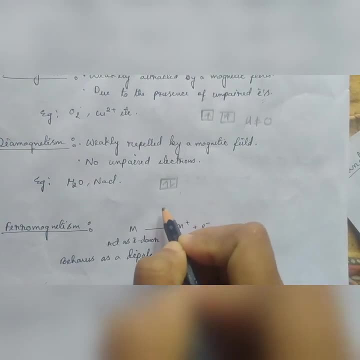 paired. paired means what one electron paired. paired means what one electron will be in a upper direction, another will be in a upper direction, another will be in a upper direction, another will be in a lower direction. so in will be in a lower direction, so in will be in a lower direction. so in diamagnetism mu will be equal to zero. diamagnetism mu will be equal to zero. diamagnetism mu will be equal to zero. that means magnetic moment will be equal. that means magnetic moment will be equal. that means magnetic moment will be equal to zero. yes, because they cancel each to zero. yes, because they cancel each. 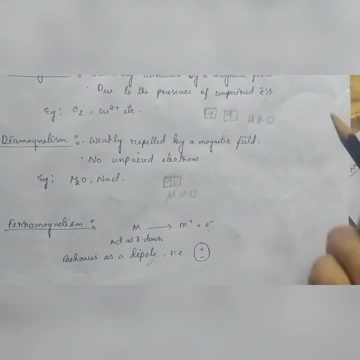 to zero. yes, because they cancel each other because both are in opposite other, because both are in opposite other, because both are in opposite direction. now, here in paramagnetism, they direction. now here in paramagnetism, they direction. now here in paramagnetism. they are weakly attracted because, in case of 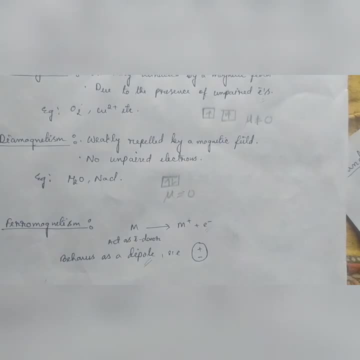 are weakly attracted because, in case of are weakly attracted because, in case of the paramagnetism, the presence of the, the paramagnetism, the presence of the, the paramagnetism, the presence of the unpaired electron is very less for unpaired electron is very less for. 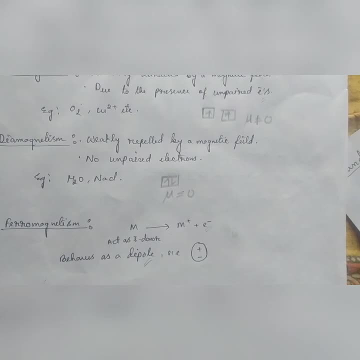 unpaired electron is very less, for example, in O2. there are only two example in O2. there are only two example in O2. there are only two unpaired electrons are there, so they are unpaired electrons are there, so they are unpaired electrons are there, so they are weakly attracted by a magnetic field. 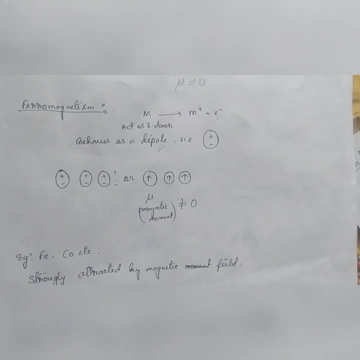 weakly attracted by a magnetic field. weakly attracted by a magnetic field now. next one is what ferromagnetism now now. next one is what ferromagnetism now now. next one is what ferromagnetism now. what happened in paramagnetism? first of, 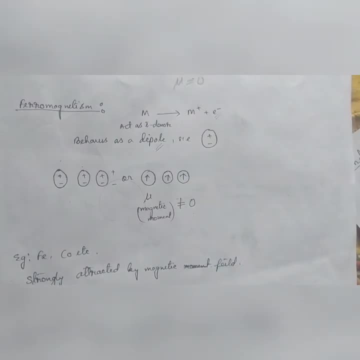 what happened in paramagnetism? first of what happened in paramagnetism, first of all, the metal. okay, the metal is act as all the metal. okay, the metal is act as all the metal. okay, the metal is act as what electron donor. that's why it will. 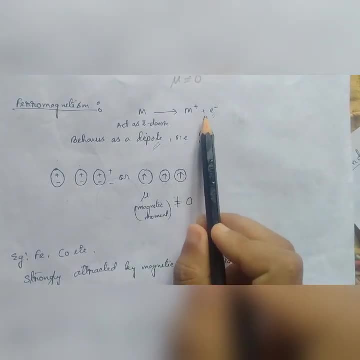 what electron donor. that's why it will. what electron donor? that's why it will. donate it's one of the electron, and with donate it's one of the electron, and with donate it's one of the electron, and with convert to what M plus plus electron. convert to what M plus plus electron. 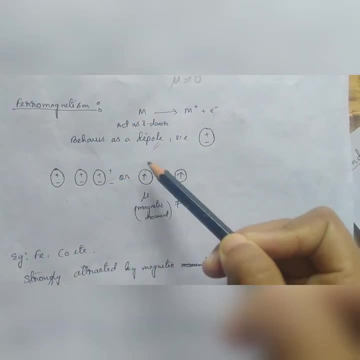 convert to what: M plus plus, electron minus. okay, that's why this metal will minus. okay, that's why this metal will minus. okay, that's why this metal will behaves as a dipole. dipole means what behaves as a dipole. dipole means what behaves as a dipole. dipole means what? where positive and negative charcer there. 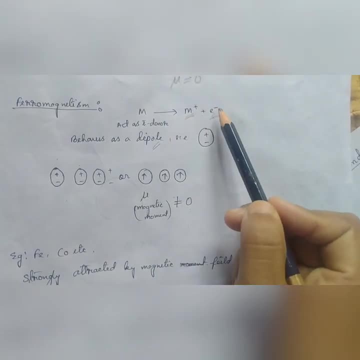 where positive and negative charcer there, where positive and negative charcer there, so in metal also M plus, that means so, in metal also M plus, that means so in metal also M plus, that means positive charge. electron minus, that means positive charge. electron minus, that means positive charge. electron minus, that means negative charge. water there so and it 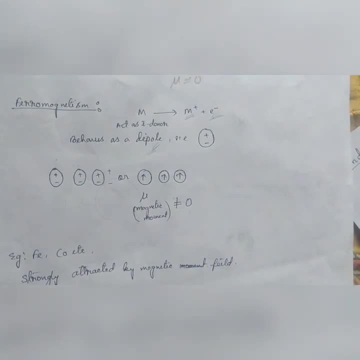 negative charge water there, so and it negative charge water there, so and it will acts as what dipole- okay now. when will acts as what dipole? okay now. when will acts as what dipole? okay now, when magnetic field is applied, then the ions. magnetic field is applied, then the ions. 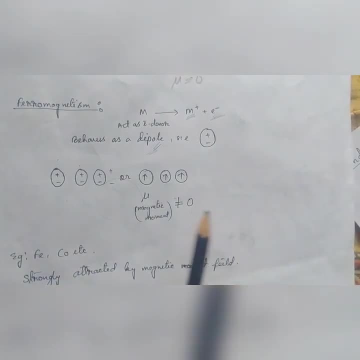 magnetic field is applied, then the ions of this metal will try to arrange. of this metal will try to arrange. of this metal will try to arrange themselves okay. and in paramagnetism they themselves okay. and in paramagnetism they themselves okay. and in paramagnetism they arrange like this: plus minus, plus, minus. 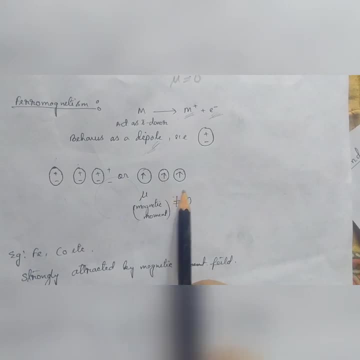 arrange like this: plus minus, plus minus. arrange like this: plus minus, plus, minus, plus minus. or in the same direction: this plus minus. or in the same direction: this plus minus, or in the same direction. this is the alignment of magnetic moment. okay, is the alignment of magnetic moment okay. 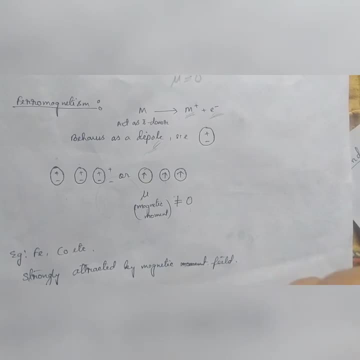 is the alignment of magnetic moment. okay, now what you done. you apply the magnetic. now what you done. you apply the magnetic. now what you done, you apply the magnetic field now. if you remove the magnetic field now, if you remove the magnetic field now, if you remove the magnetic field from this ions, then also the group. 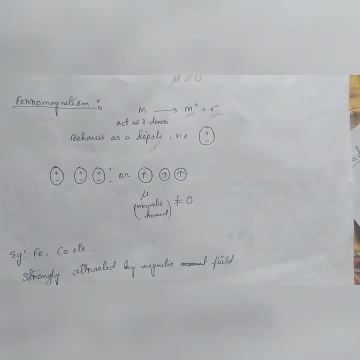 field from this ions, then also the group field from this ions, then also the group of this ions will act as a teeny magnet of this. ions will act as a teeny magnet of this. ions will act as a teeny magnet. okay, they convert to the permanent. 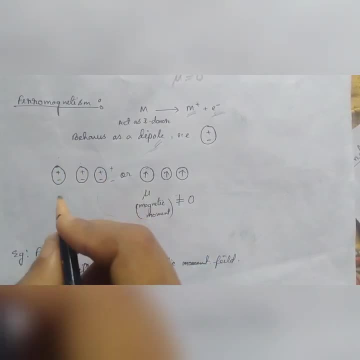 okay, they convert to the permanent. okay, they convert to the permanent magnet. okay, so these are known as what magnet? okay, so these are known as what magnet. okay, so these are known as what? domains means the group of ions they act. domains means the group of ions they act. 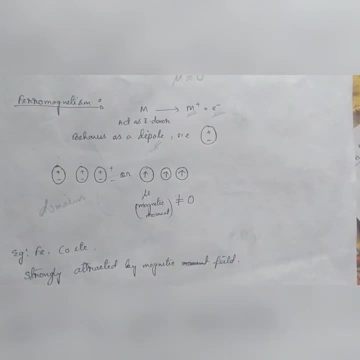 domains means the group of ions they act, which acts as a teeny magnet because we. which acts as a teeny magnet because we. which acts as a teeny magnet? because we applied here the magnetic field, so this applied here the magnetic field, so this applied here the magnetic field. so this group of ions are known as what domains? 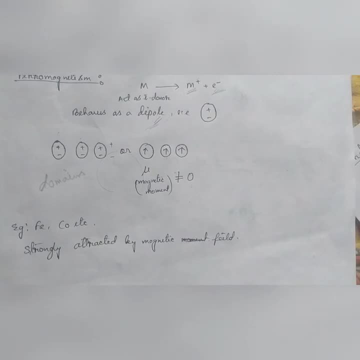 group of ions are known as what domains group of ions are known as what domains? okay and exemplar iron cobalt, etc. and okay and exemplar iron cobalt, etc. and okay and exemplar iron cobalt, etc. and this substances are strongly attracted by this. substances are strongly attracted by. 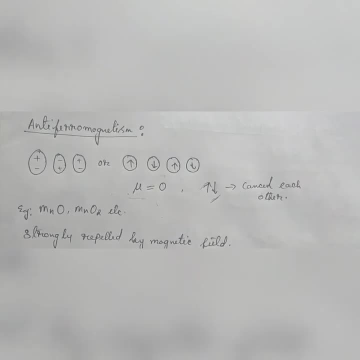 this: substances are strongly attracted by a magnetic field. so next one is: what a magnetic field? so next one is: what a magnetic field? so next one is: what anti ferromagnetism? so in anti, anti ferromagnetism, so in anti, anti ferromagnetism, so in anti ferromagnetism. the domains are arranged. 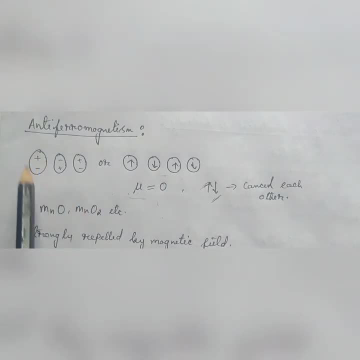 ferromagnetism: the domains are arranged. ferromagnetism: the domains are arranged in this way, okay, in a proper way. plus, in this way, okay, in a proper way. plus, in this way, okay, in a proper way. plus, minus, minus. plus, plus, minus, that means minus, minus. plus, plus, minus, that means. 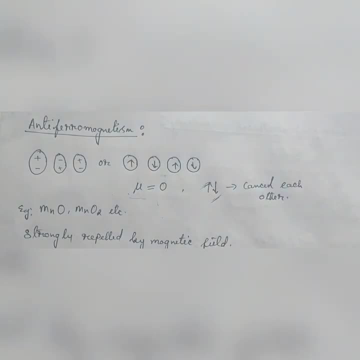 minus minus, plus plus minus. that means, like this one will be in a upper side. like this one will be in a upper side. like this one will be in a upper side, another will be in a lower side, upper. another will be in a lower side, upper, another will be in a lower side, upper side, lower side. like this in a range, in a. 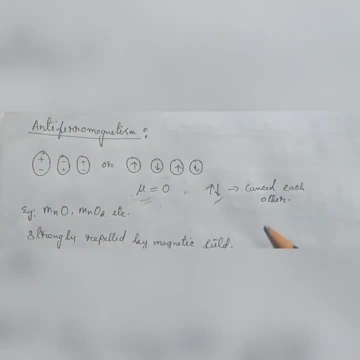 side, lower side, like this in a range, in a side, lower side. like this in a range, in a range, in a range in a proper way. okay, so here the proper way. okay, so here the proper way. okay, so here the change in magnetic moment will be equal. 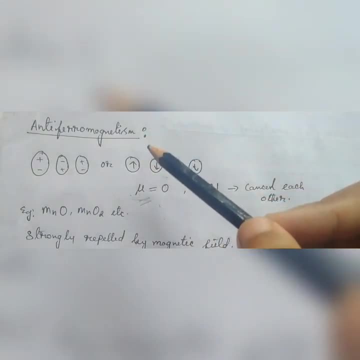 change in magnetic moment will be equal. change in magnetic moment will be equal to 0, because they will cancel each other to 0. because they will cancel each other to 0, because they will cancel each other. one is in upper side, this will cancel. one is in upper side, this will cancel. 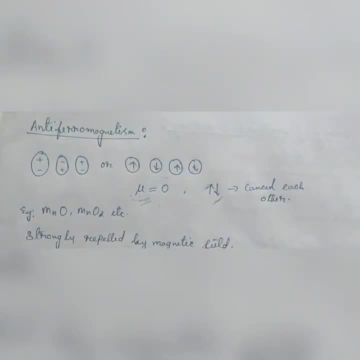 one is in upper side. this will cancel this. this will cancel this. this will this. this will cancel this. this will this. this will cancel this. this will cancel this. like this. okay, they will cancel this like this. okay, they will cancel this like this. okay, they will cancel each other. that's why this. 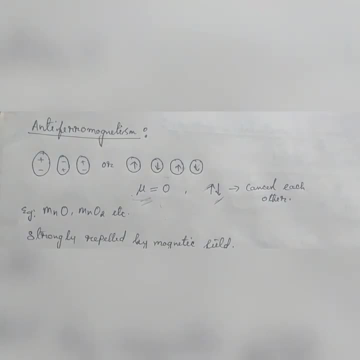 cancel each other. that's why this cancel each other. that's why this magnetic moment will be zero in magnetic moment, will be zero in magnetic moment, will be zero in antiferromagnetism- okay, and these are antiferromagnetism okay, and these are antiferromagnetism okay, and these are strongly repelled by a magnetic field. 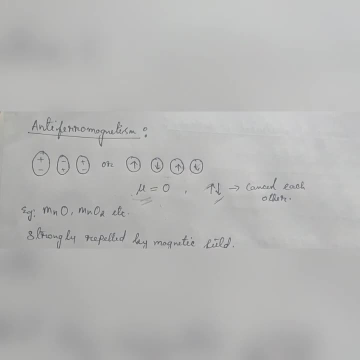 strongly repelled by a magnetic field. strongly repelled by a magnetic field. examples are like manganese oxide. examples are like manganese oxide. examples are like manganese oxide, manganese dioxide, etc. okay, and the last, manganese oxide, manganese dioxide, etc. okay, and the last, manganese oxide, manganese dioxide, etc. okay, and the last one is very magnetism. so in 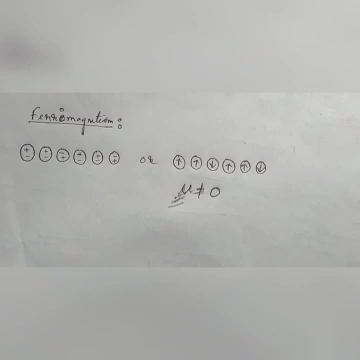 one is very magnetism, so in one is very magnetism. so in ferrimagnetism the domains are not ferrimagnetism, the domains are not ferrimagnetism, the domains are not arranged in a proper way. okay, the arranged in a proper way, okay, the. 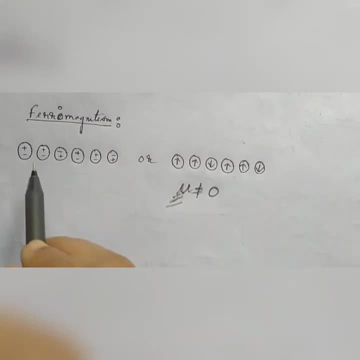 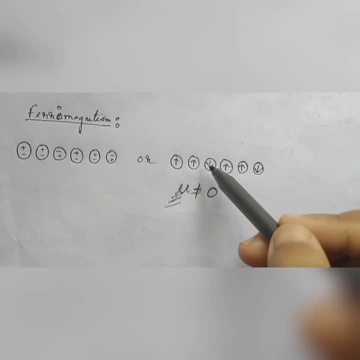